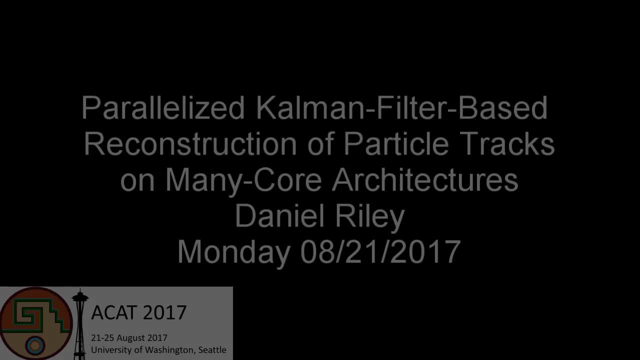 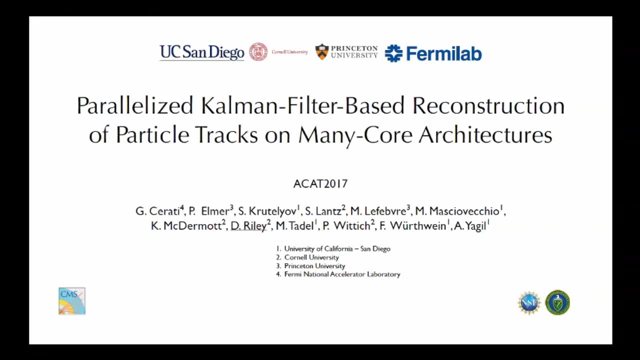 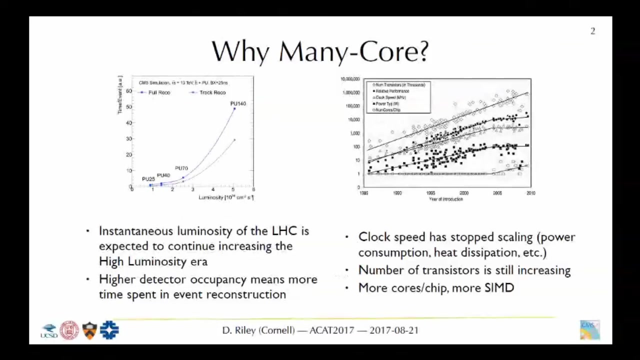 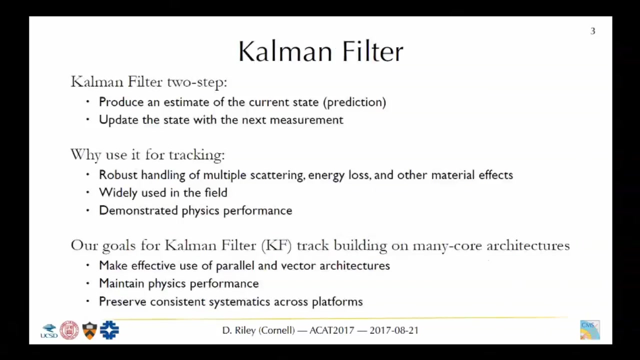 And so the last talk we'll do will tell us about parallelization of the common filter, and the speakers stand by. So this project is looking at parallelizing vectorized common filter. Why are we doing that and what's it for? Well, you heard about common filter this morning. 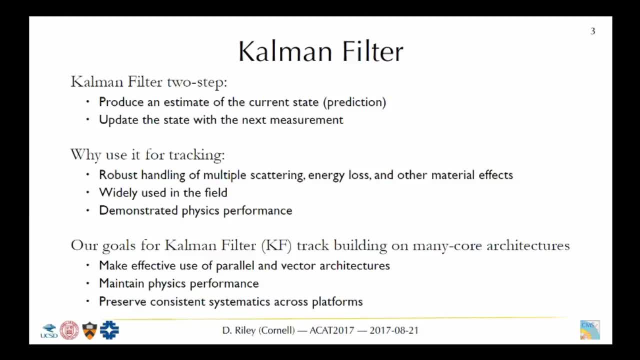 It's basically a way of producing an estimate of a track that is in some sense optimal, Basically by adding new information as you pop up in the track through this detector. And why It's effective for tracking? because it gives you a robust handling of multiple scattering. 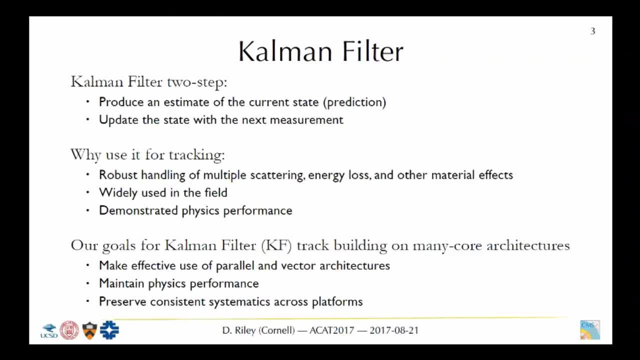 energy loss and material effects. It's widely used. We've spent, you know, decades understanding its performance. So our goal is to try and make effective use of parallel vector architectures, common filter, maintain the physics performance. That means, in particular, we want to try and maintain consistency across platforms. 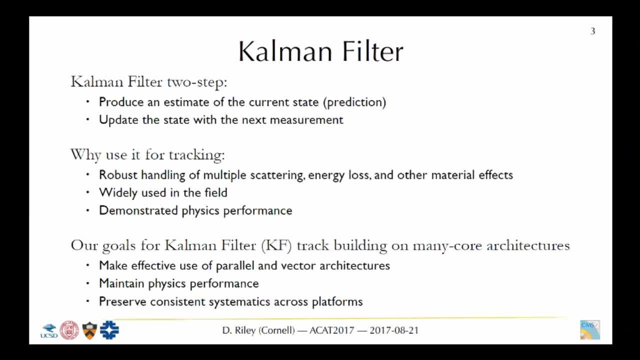 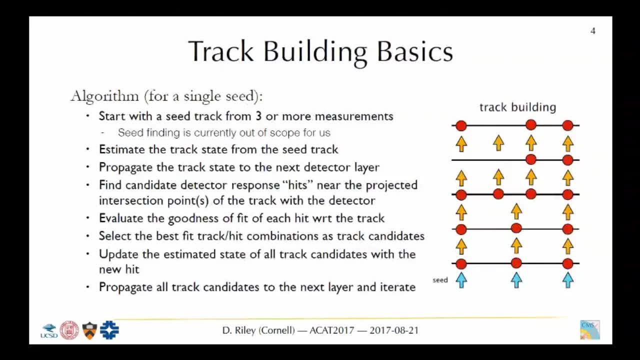 We want to be able to. We want to take the opportunistic use of different kinds of unconventional architectures Which may be over the ambitious. So the basics of track building: you start from a set of seeds and finding seeds is out of scope for us. 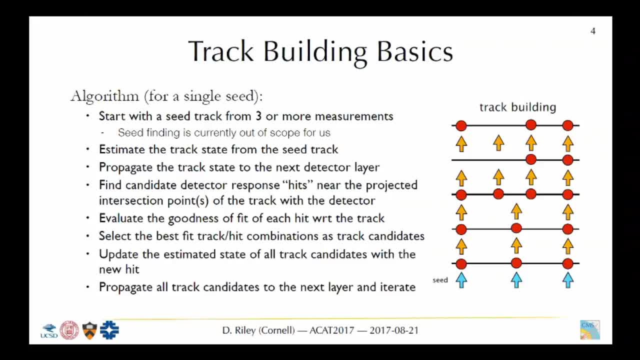 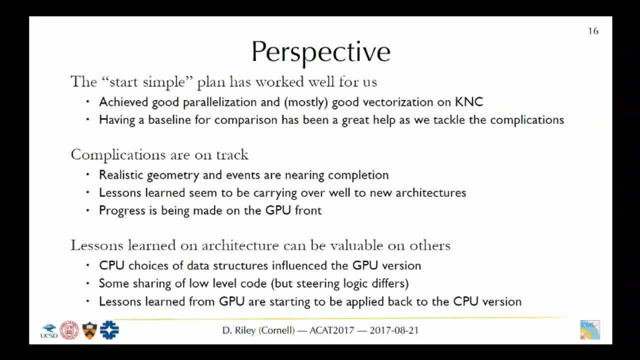 Once you've got that, you're going to start to think about what's the best way to do that. Once you've got that, you're going to start to think about what's the best way to do that. It's because it's it's. that's all the common filter map is it's you're taking. 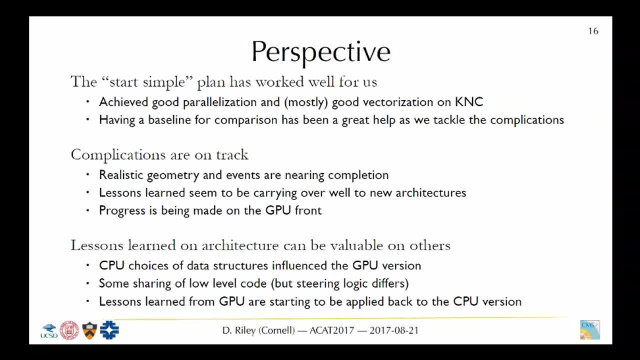 a track state this: six vectors, three spatial, three momentum coordinates and propagating. in the next layer we need a Jacobian. the cross product of those assists, that's a six by six, and everything in the propagation station is those six coordinates and one by six. yeah, yes, so that was the g-flex, is the? is the gpu version of the structure. so